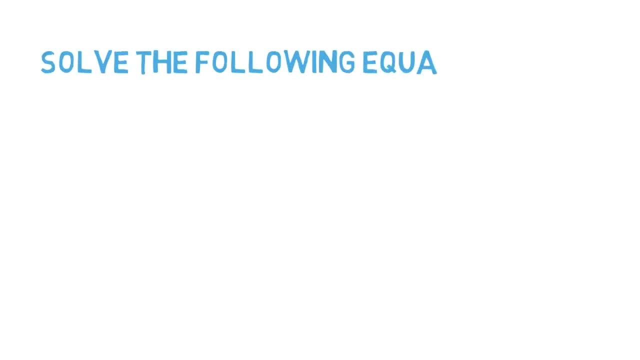 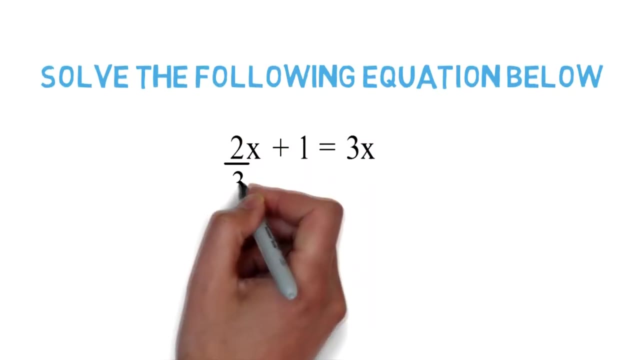 Solve the following equation below, and you're given: two thirds x plus one half equals three fourths x. Now, at this second, I'd like you to please pause this video and try it out yourself so you see if you get it right. see what mistakes you made, And one of the first. 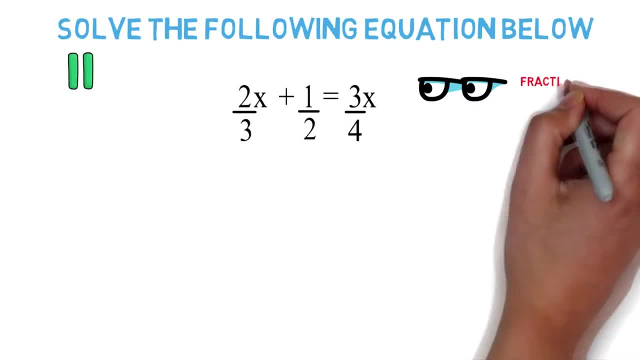 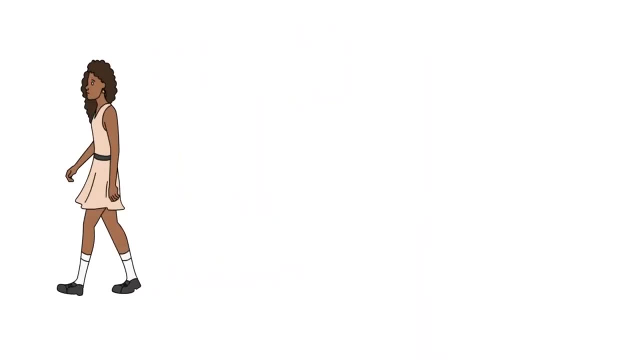 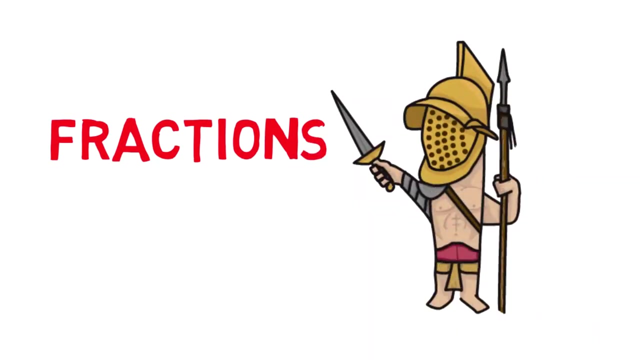 things you should notice is that this is a fraction type equation problem. So here is one example of some steps you can use to solve this problem, and it begins with the first step, which is to eliminate the fractions. And some teachers say: fractions are your friend, but what you should do is you should eliminate. 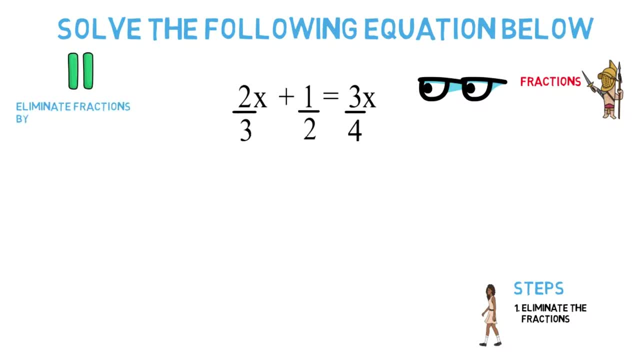 these fractions. you should fight them at any chance you get. So how do you eliminate the fractions? Well, you can eliminate fractions by multiplying the equation by the least common multiple of the denominator. Which brings us to our question: what is the least common? 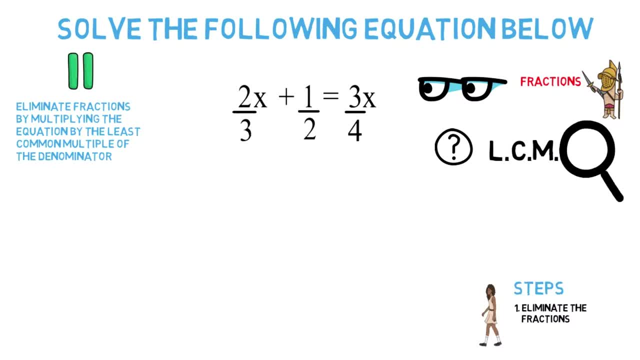 multiple of the denominators. So let's quickly investigate that And what you can do is string out multiples of the denominators. starting with 2, which gives you 2,, 4,, 6,, 8,, 10, 12.. 3 is 3,, 6,, 9,, 12,, 15.. 4, you get 4, 8,, 12,, 16.. And you'll notice. 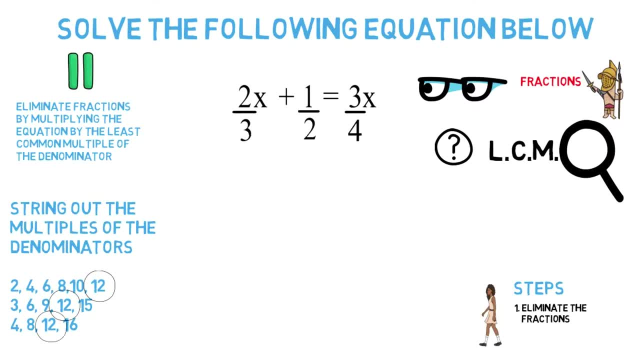 that the common multiple is going to be 12 as it comes up in all three strings. So our least common multiple will be 12.. And now what you're going to do is you're going to take that 12 and you're going to multiply it to both sides of the equation, or basically just multiply. 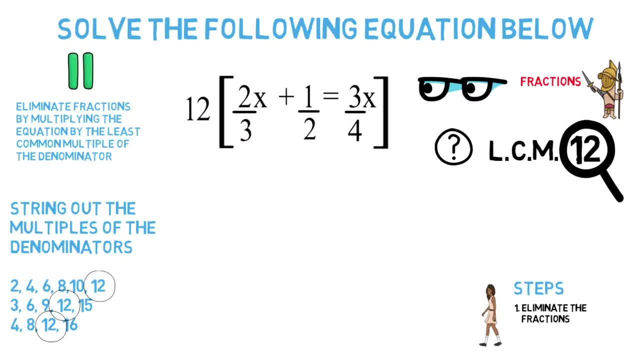 it to every term in the equation, And the reason we're multiplying everything by 12 is so that we can divide out and eliminate these fractions. You'll do 12 divided by 3, which will give you a 4.. And then you'll take that 4 and you're going to multiply it by 2x.